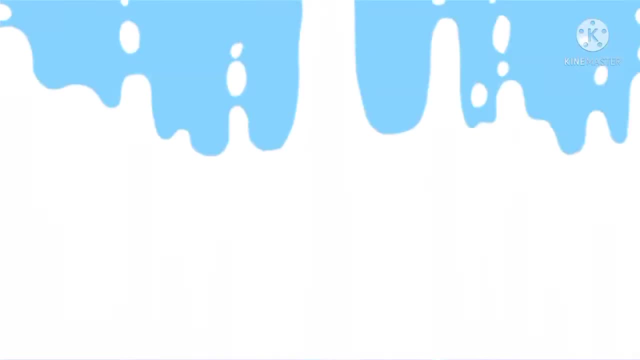 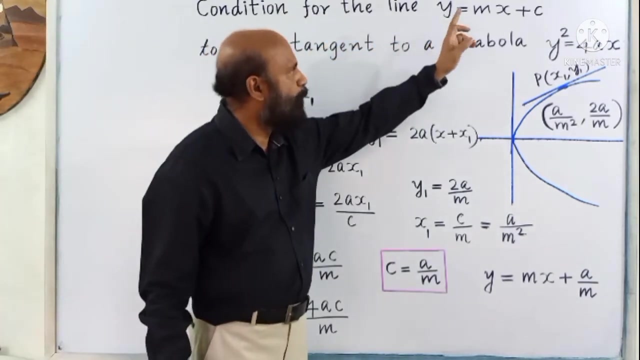 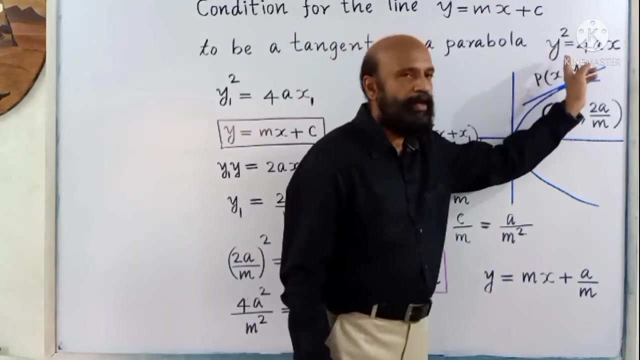 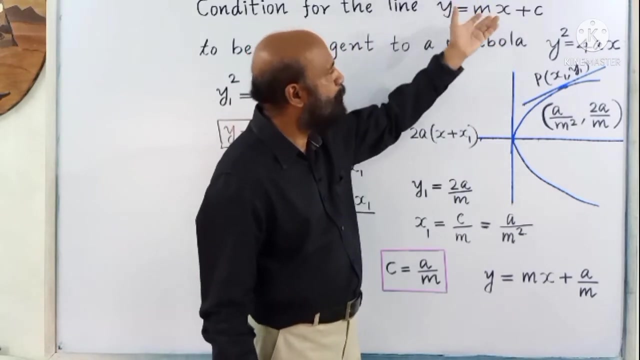 In this video. let us see the condition for the line y is equal to mx plus c to be a tangent to a parabola. The equation of the parabola is: y square is equal to 4ax, Then you have to get the condition for this line to be a tangent. 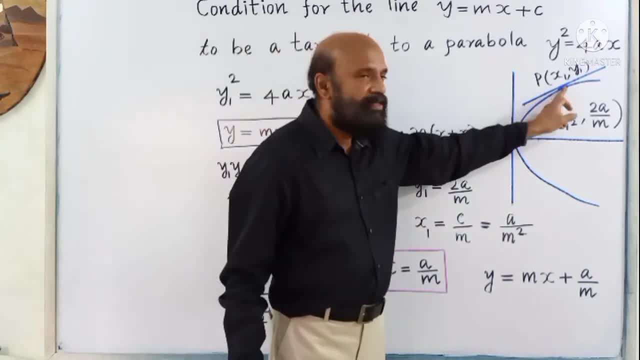 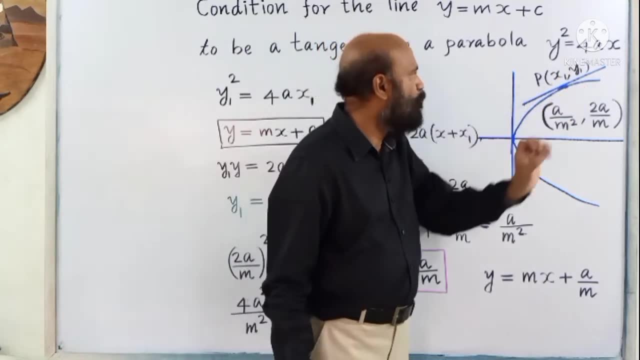 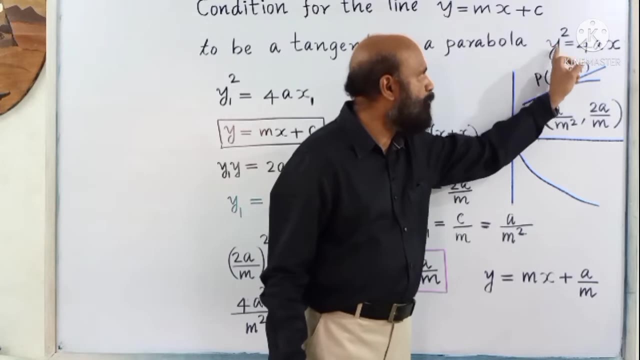 Let p be a point on the parabola. Its coordinates x1 comma y1.. Since the point is on the parabola, it should satisfy the equation of the parabola. Equation of the parabola is: y square is equal to. 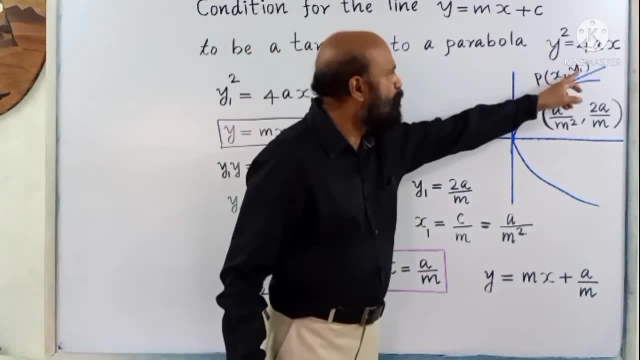 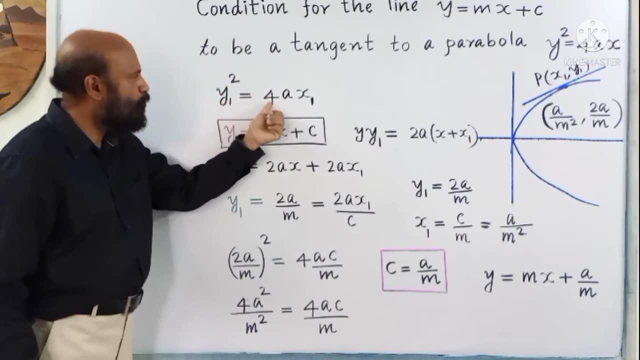 4ax. So instead of y you have to put y1. Then instead of x, x1.. So it should satisfy the equation of the parabola. So we can write: y1 square is equal to 4ax. Our aim is to find the condition for the line y is equal to mx plus c to be a tangent to this. 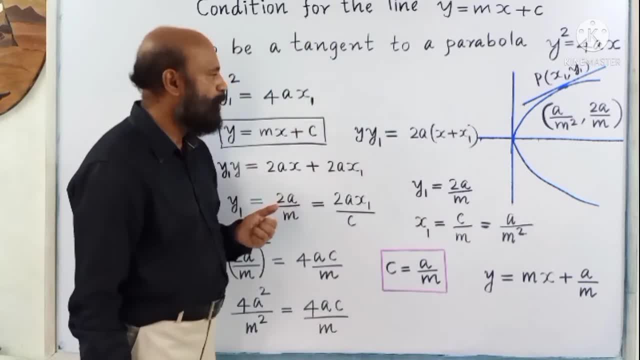 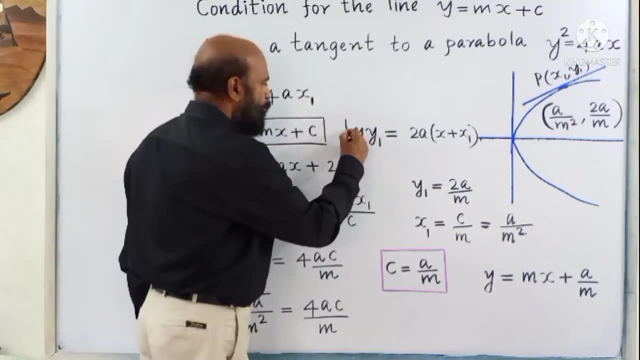 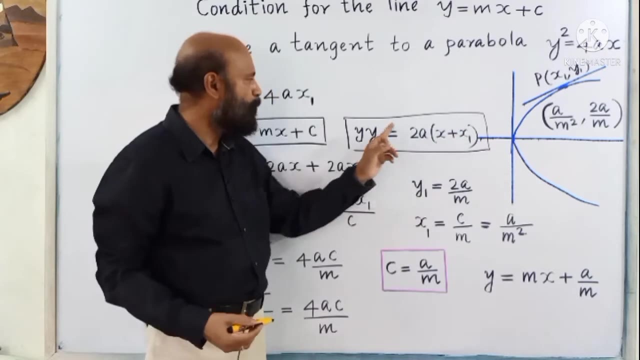 parabola. You know the equation of a tangent at the point x1 comma y1.. This is the equation: yy1 is equal to 2a into x plus x1.. So this is the equation of a tangent at the point x1 comma y1. 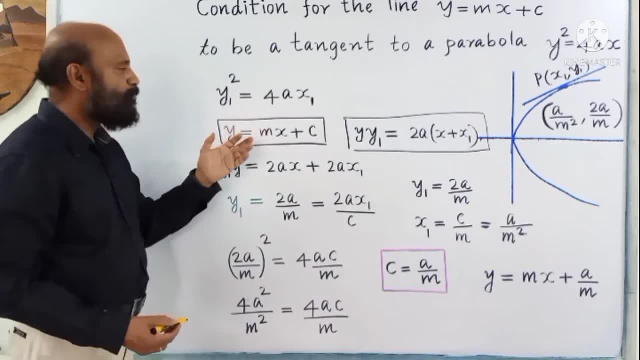 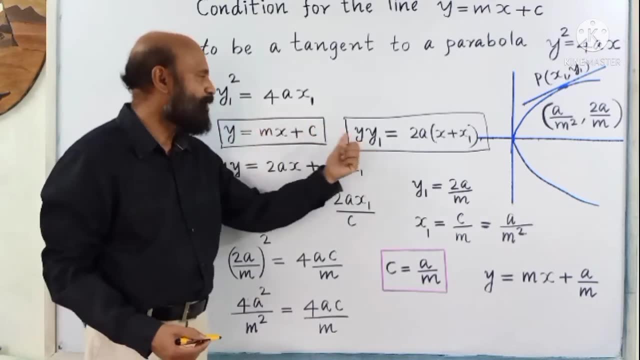 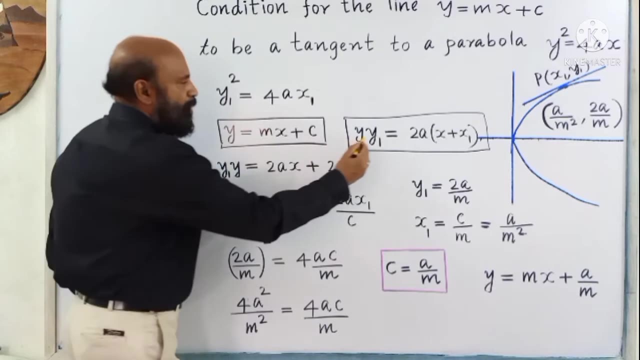 If this is to be the tangent, then coefficients should be proportional. Now these two are representing the same line, So you rearrange this So we can write y1y, Then, after removing the bracket, 2ax plus 2ax1.. 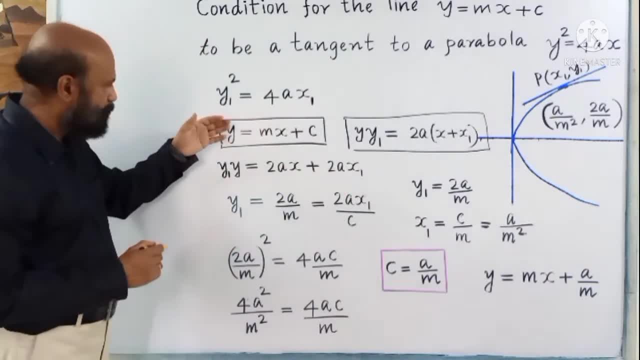 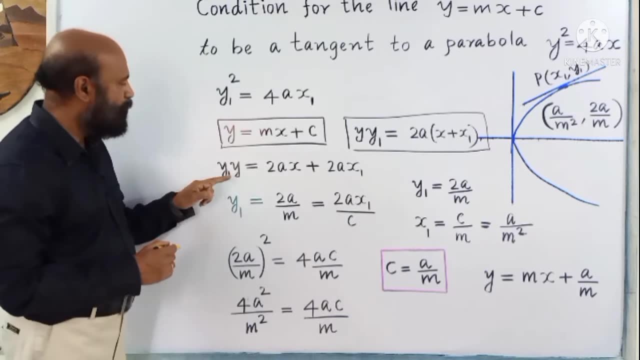 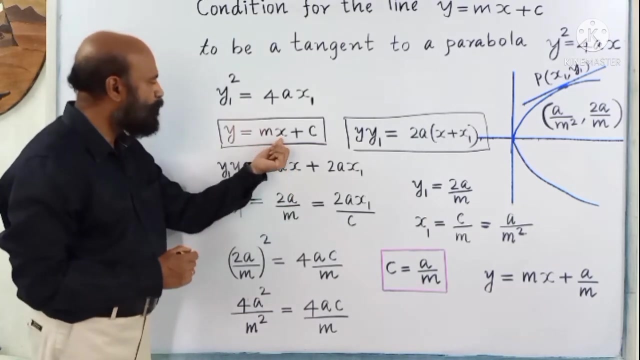 Now these two are representing the same lines. Then coefficients should be proportional. So now, here coefficient of y is y1.. Here coefficient of y is 1.. So y1 by 1 is equal to. here coefficient of x is 2a. Here coefficient of x is m. So y1 should be equal to 2a by m. 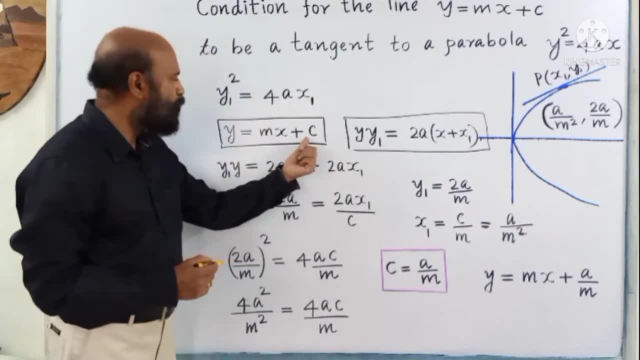 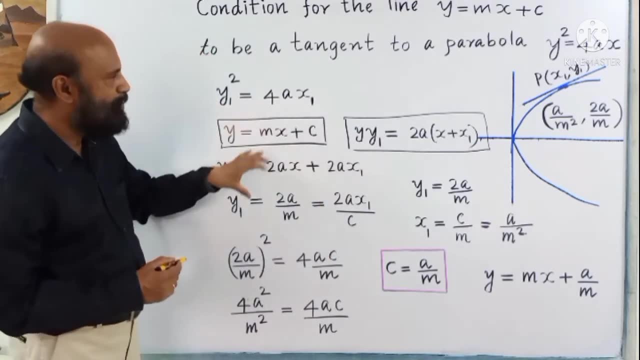 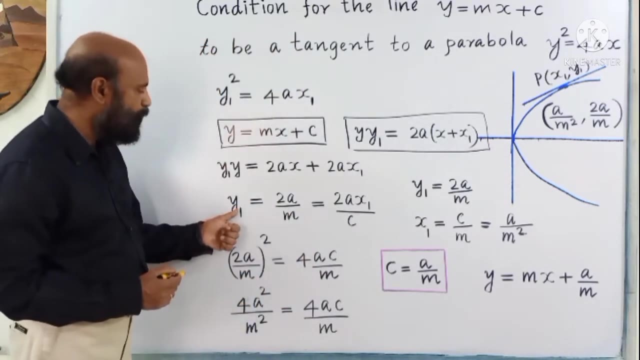 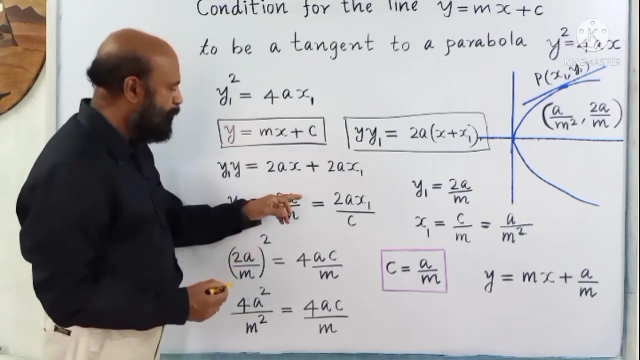 Then here constant is 2ax1.. Here constant is c, So 2ax1 by c. Since these two lines are representing same lines, coefficients should be proportional. From this we can write: y1 is equal to 2a by m, Then x1 will be c by m. This 2a and this 2a. 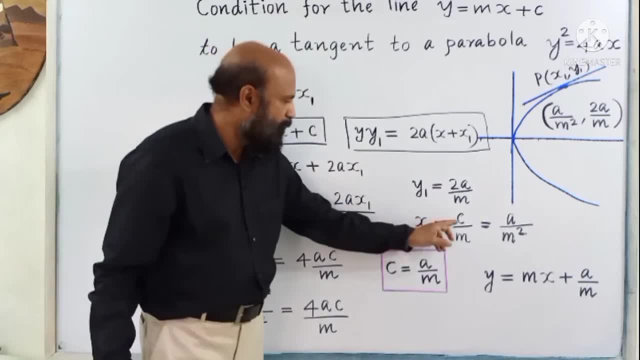 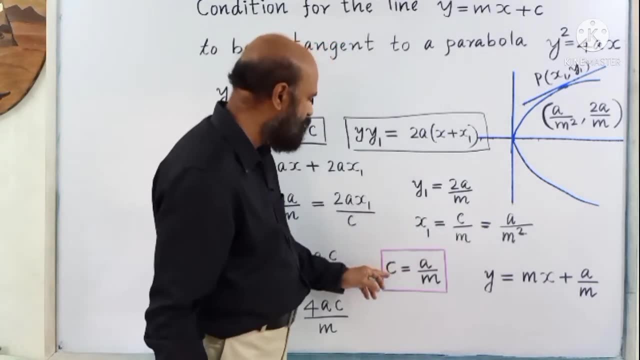 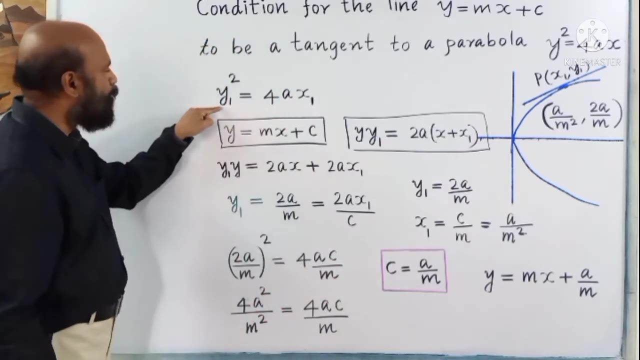 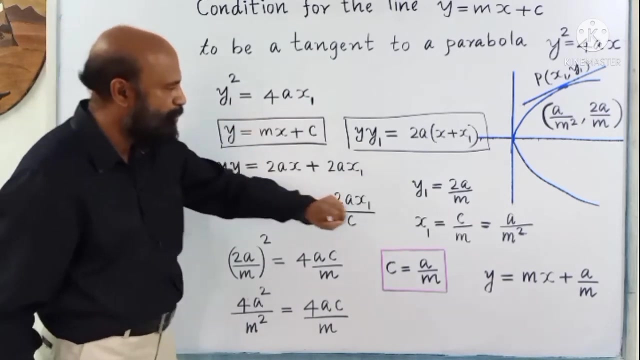 will get cancelled, So you can write x1. is c by m, Then for this c should be a by m That we can get after substituting. Now, instead of this y1, you can substitute 2a by m Instead of this x1,. you can substitute c by m Instead of this x1, we can write c by m. 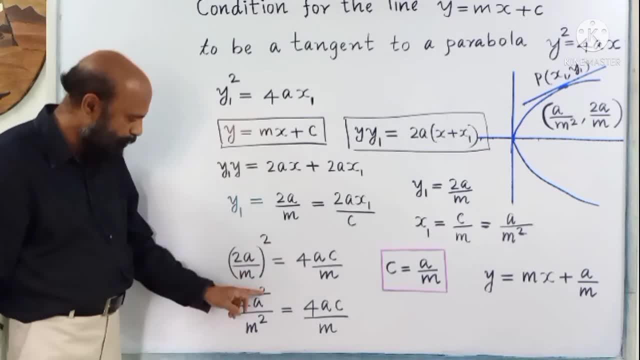 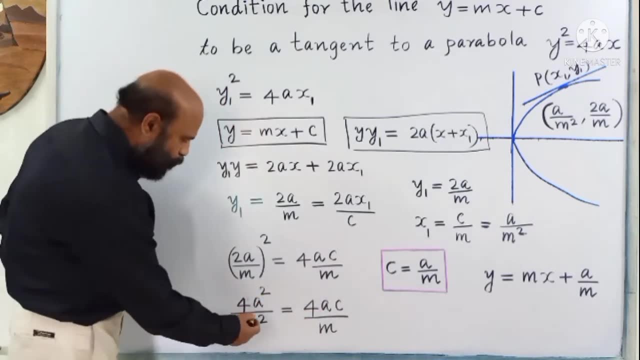 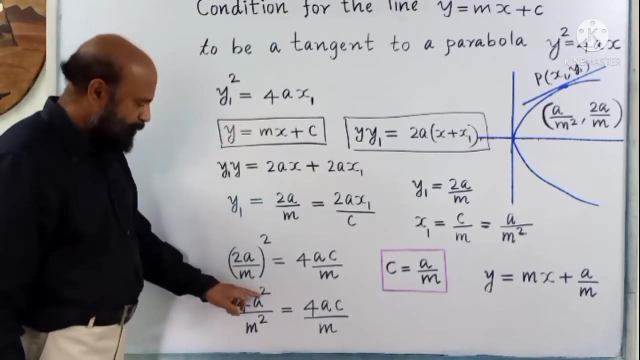 Now squaring, So it will become 4a. square by m. square is equal to 4ac by m. Now 1m will get cancelled. Here m square 1m will get cancelled and 4a and 4a get cancelled. 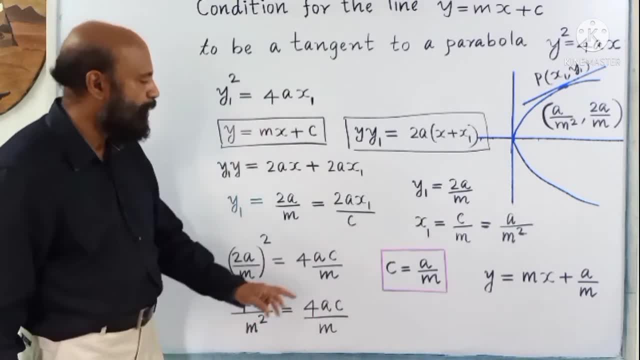 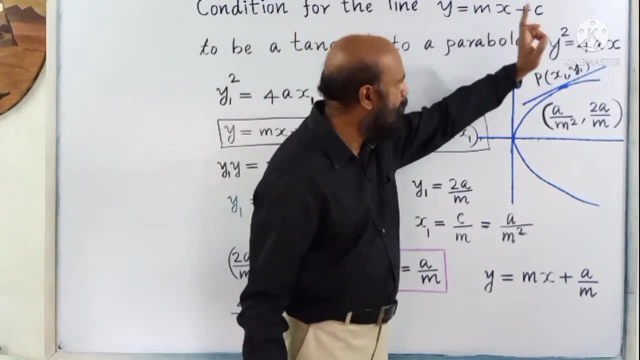 So here there will be 1a, So c should be a by m. So this is the condition: If this line, y is equal to mx plus c is to be a tangent to the parabola. y square is equal to 4ax, c should be a by m. 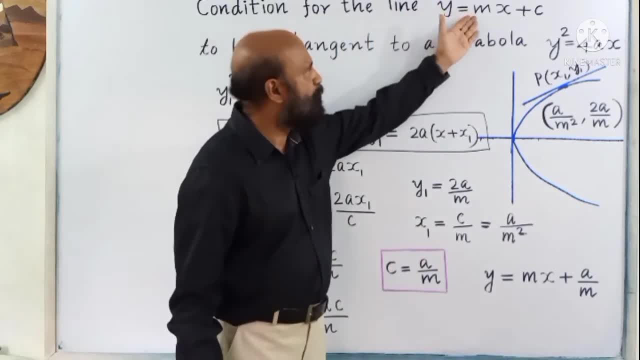 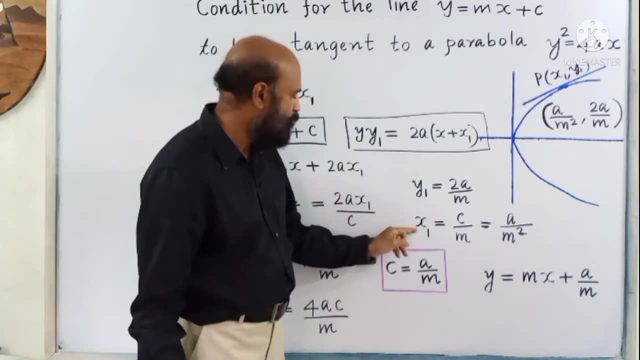 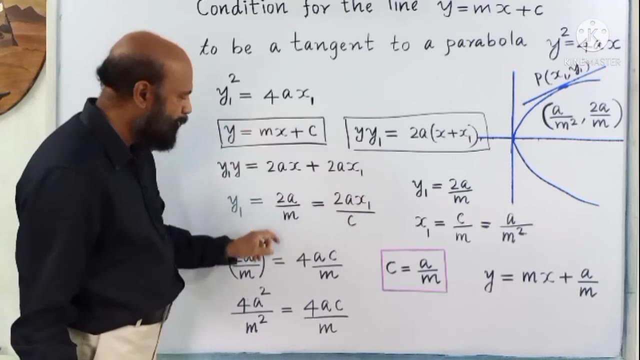 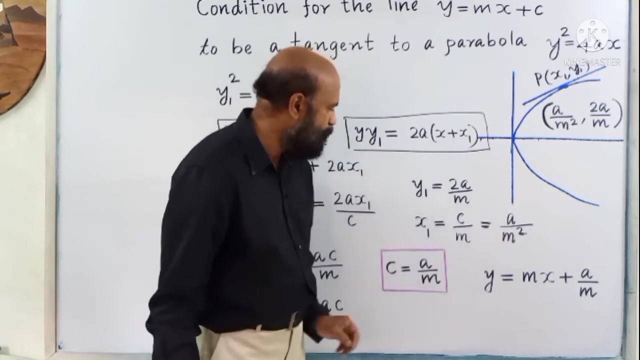 This is the condition. Then this line will become a tangent Now point of contact. So point of contact is: x1 is c by m That you can get from this 2a after cancellation. x1 is c by m, But for c we can write a by m, So it will become a by. 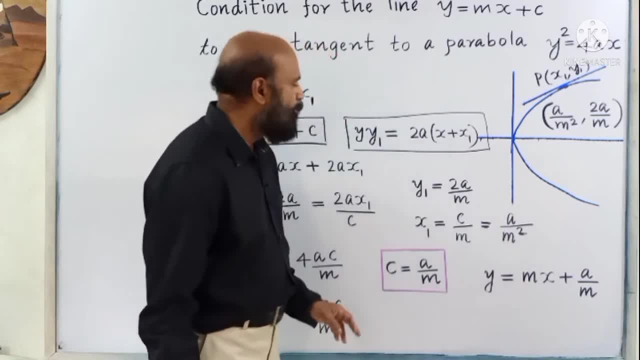 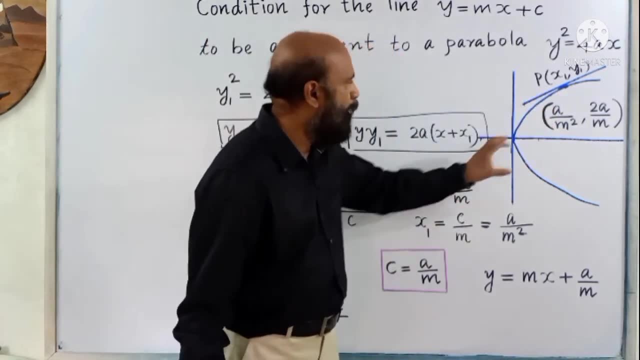 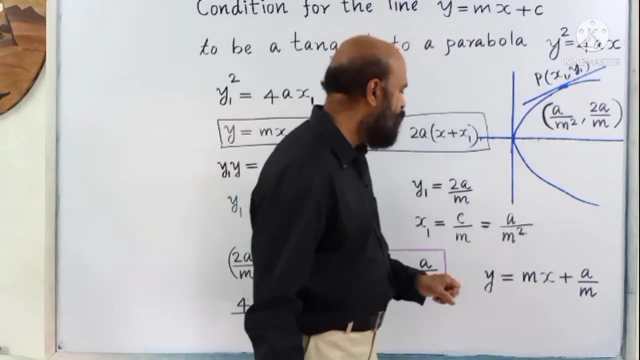 this m is there, So a by m square. So the points of point of contact. Point of contact is a by m square and 2a by m. x1 is a by m square and y1 is 2a by m. then y is equal to mx plus c, since c is a by m. 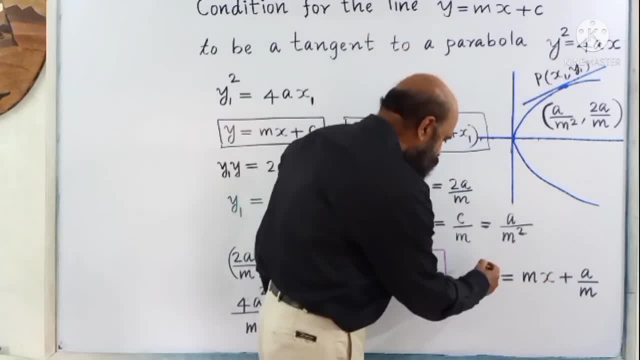 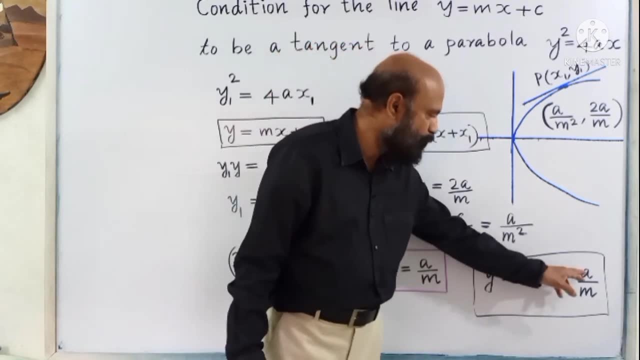 so you can write. for the c, we can write. so this is the equation of the tangent: y is equal to mx plus c, but instead of c we can write a by m.